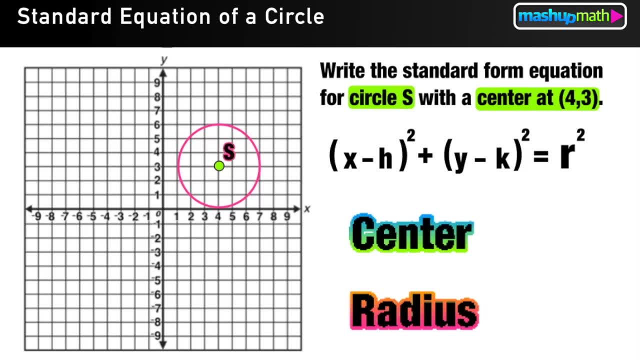 and the length of its radius. Now the question already told me that at point S is the center, at 4, 3.. So I'm already half done with what I need Now to find the radius. I'm going to start at the center, at point S, and draw a line that goes directly to the edge of the 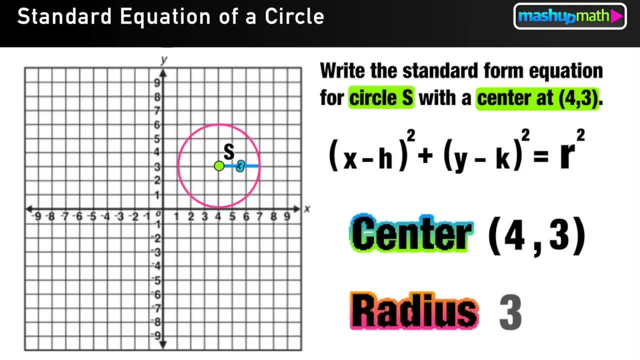 circle and then count the number of units, in this case 3.. Now it's okay if you count it in a different direction, since we know that all radii are the same length, all are going to be 3.. So, now that we have the center and the radius, we have the information that 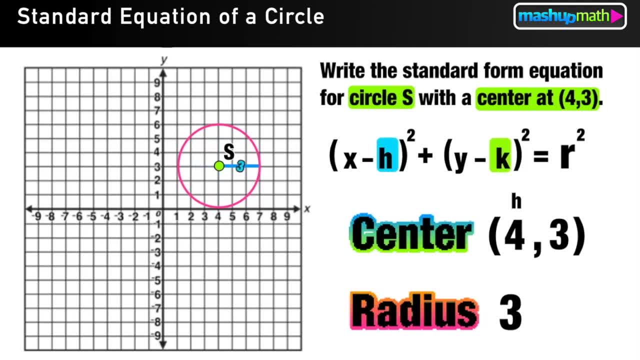 we need to write the equation of this circle. We know h and k now. h is the x coordinate, k is the y coordinate, so h is going to be replaced with the number 4, and k will be replaced with the number 3.. And since the radius of circle S was 3,, replace the r with. 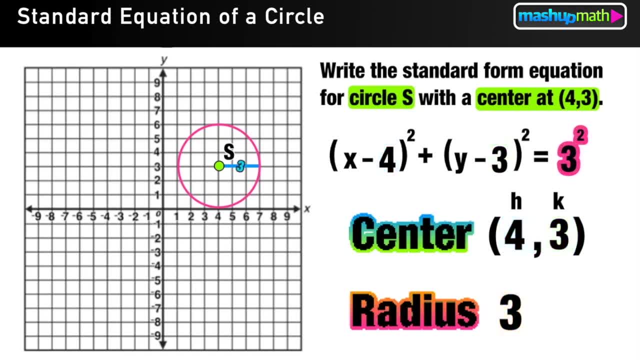 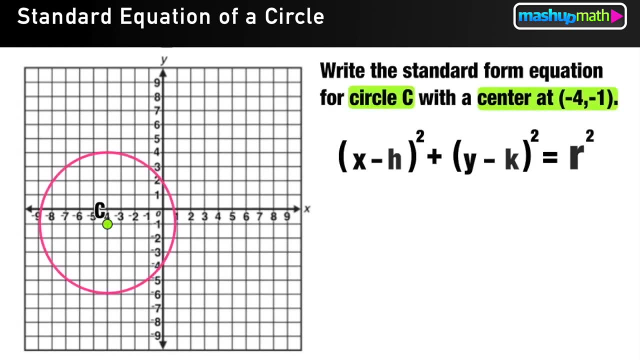 r squared with 3 squared and of course, 3 squared evaluates to positive 9, and now we have the standard form equation of circle S. So for our second example, again, we want to write the standard form equation for circle C with a center at negative 4, negative 1.. So the information that we need to answer: 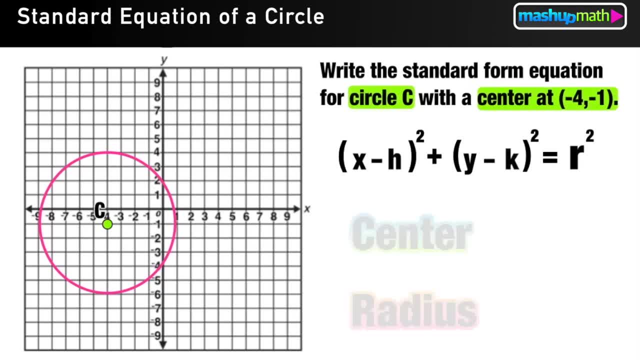 this question is the location of the center of the circle and the length of its radius. Now we already know that C is the center and has coordinates at negative 4 and negative 1, and to find the radius we start from C and count right to the edge of the circle. 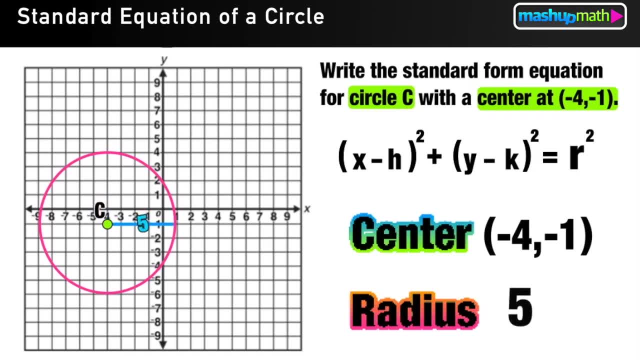 in this case 5 units, so our radius is 5.. So now we're ready for the equation. We're going to go ahead and replace the h with negative 4, and the k with negative 1, and replace r squared with 5 squared. Notice that x minus negative 4, the double negative becomes a. 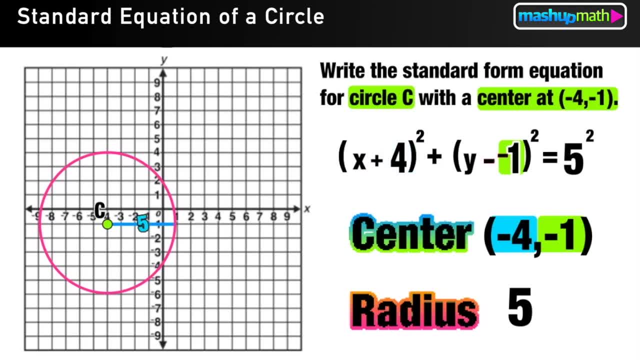 positive, so we have x plus 4.. And the y minus negative 1 becomes y plus 1.. So, effectively, what we're doing is just switching the sign: negative becomes positive, and positive becomes negative, And finally we know that 5 squared is equal to 25, and now we have our standard form equation. 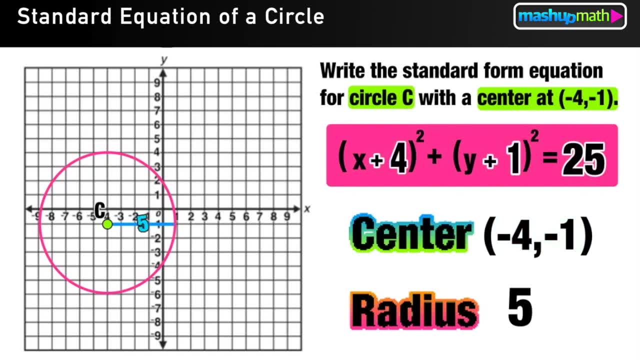 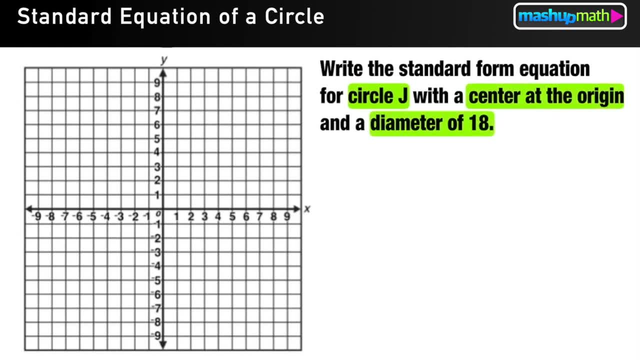 of circle C. This next example wants us to write the standard form equation for circle J, with a center at the origin and a diagonal. So in the same line of thinking, here we know that we're going to need to fill out the standard form equation of a circle, which means that we're going to need a center, n radius. Now 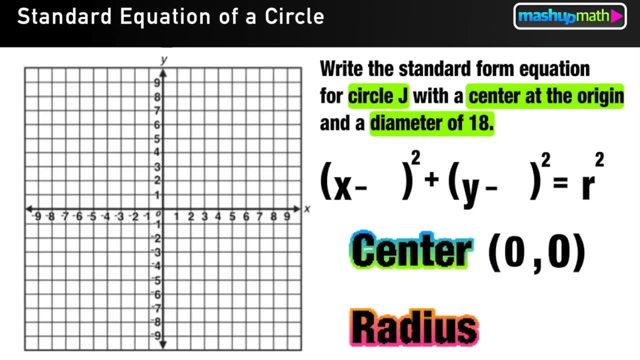 the question told us that the center of circle J is at the origin, which is the point. Now we'll plot that point and construct the circle so that we can visualize what's going on here. Now, the diameter is 18,, which means that the radius is going to be half of 18, which we 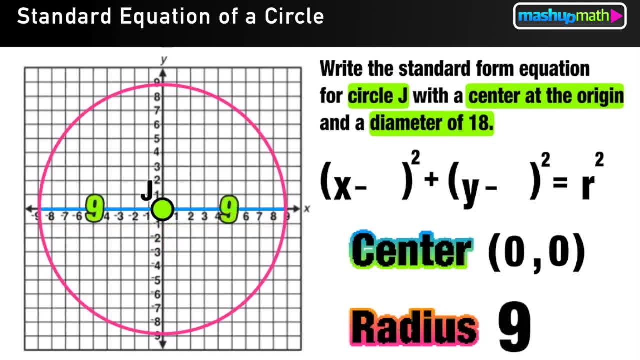 know is 9.. So now we know what this circle looks like And we have the information that we need, So I can go ahead and plug in the zeros for the x and y coordinates of the center and replace the radius value with 9.. 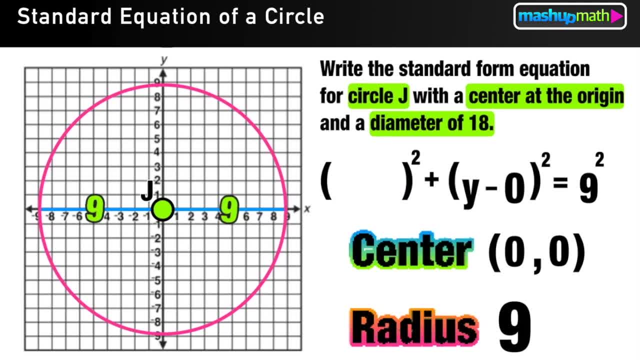 Now notice on the left side that x minus 0 is just x, so I'm not going to write it as x minus 0, I'm just going to write it as x which, when raised to the second power, is just x squared. 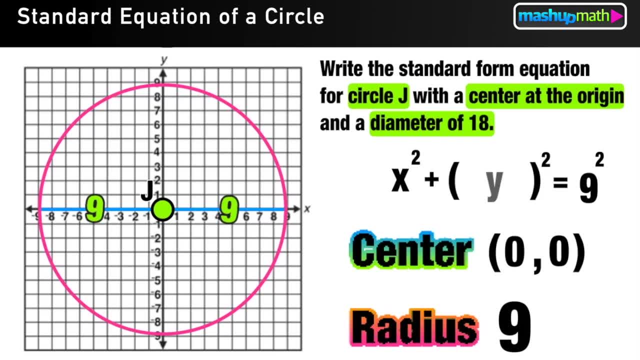 And I'm going to do the same thing with the y value: Y minus 0 is just y, and y raised to the second power is just y squared. And finally, we're going to do the same thing with the y value: y minus 0 is just y, and y raised to the second power is just y squared. 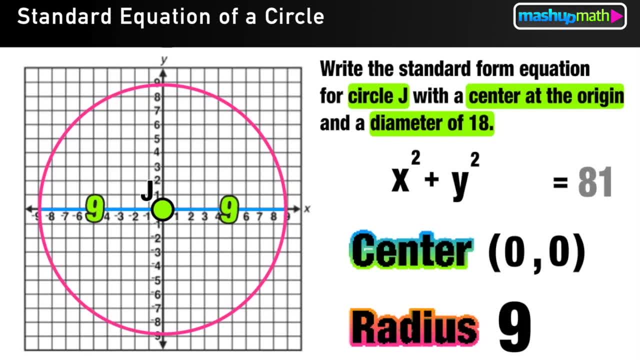 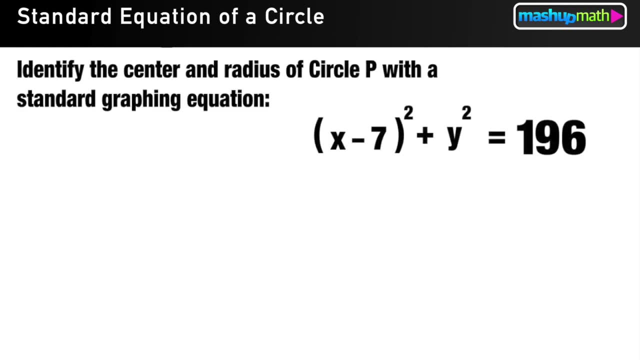 And finally, 9 raised to the second power, or 9 squared equals 81. So the equation of this circle is just: x squared plus y squared equals 81.. Now this last example is kind of like the reverse of what we have been doing. 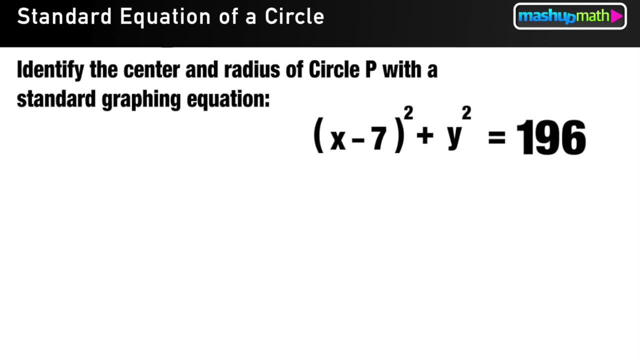 So in this question we want to identify the center and radius of a circle and it's giving us the equation. So basically, we should be thinking: if we have the equation of a circle, how do we pull from it? We should be thinking about the coordinates of the center of the circle and the length. 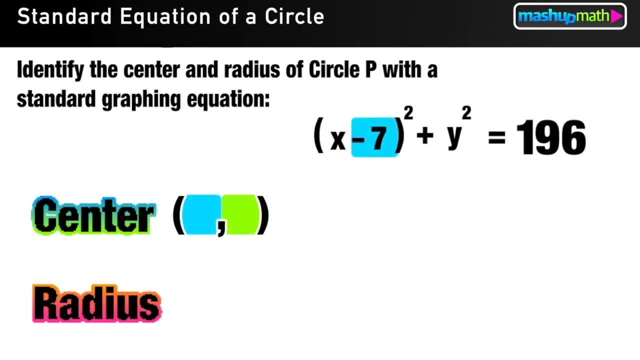 of the radius. Now the x coordinate of the center is that h value with the sign changed. So the negative 7 in the formula means that the center x coordinate is going to be positive 7.. For the y coordinate: there is no value there like in the last example. so we know it's.